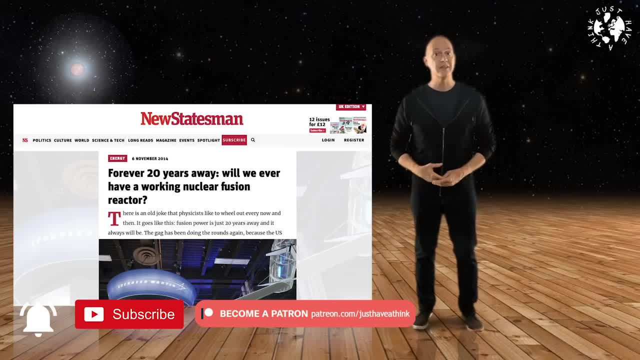 another interesting concept. it's an incredibly complex and challenging concept to bring into reality And if it was almost literally anything else, the scientists, engineers and investors would have given up long ago. Nuclear fusion is just another interesting technology. It really does offer the possibility. 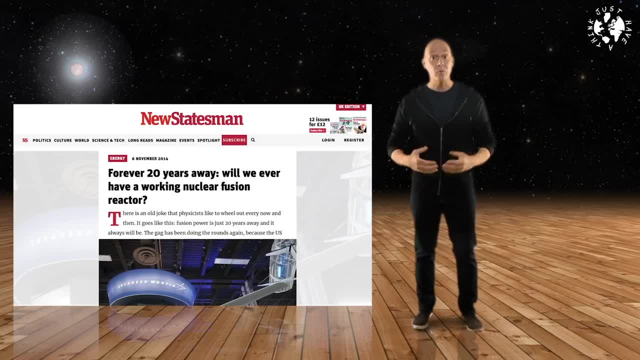 of unlimited, risk-free, zero carbon, zero waste energy for the foreseeable future of mankind, And that's a pretty compelling reason to keep persevering despite almost overwhelming odds against success. Nuclear fusion is sort of the opposite of nuclear fission, which is the process. 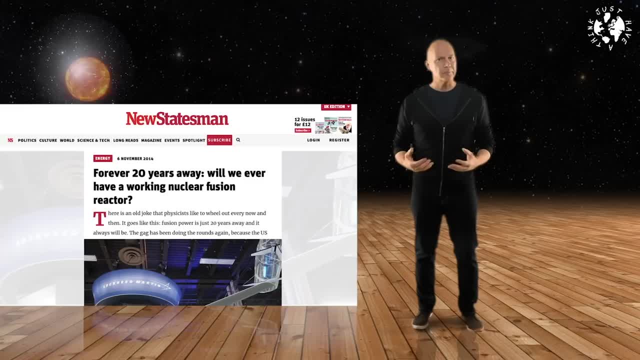 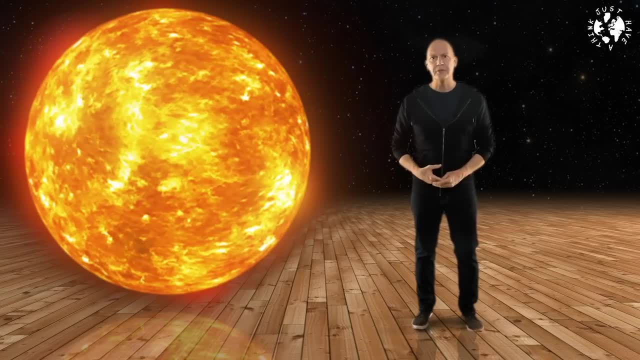 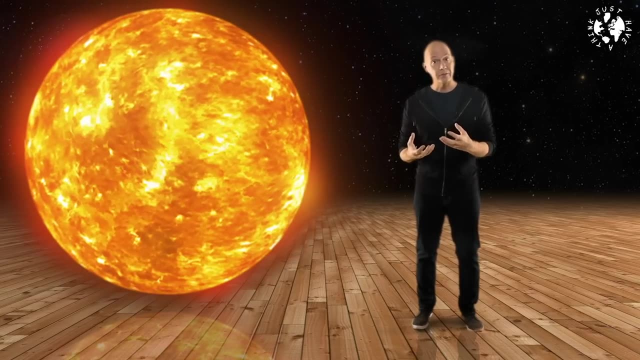 that currently drives the world's nuclear power plants. It's the process that's been powering our local star for more than four thousand million years. The enormous temperatures inside the sun strip atoms of their electrons, and that results in a plasma with atomic nuclei and electrons that are all flying around independently of each other. 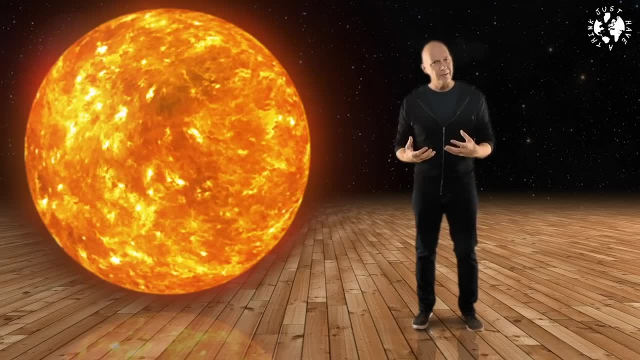 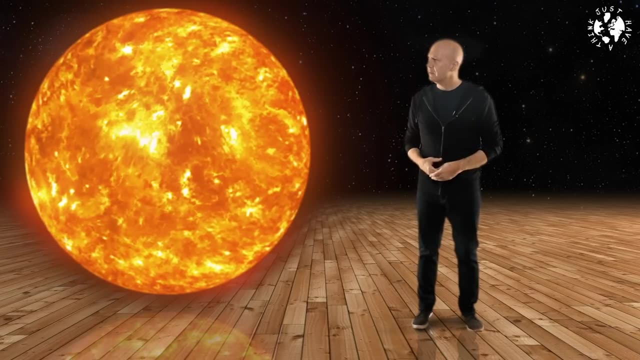 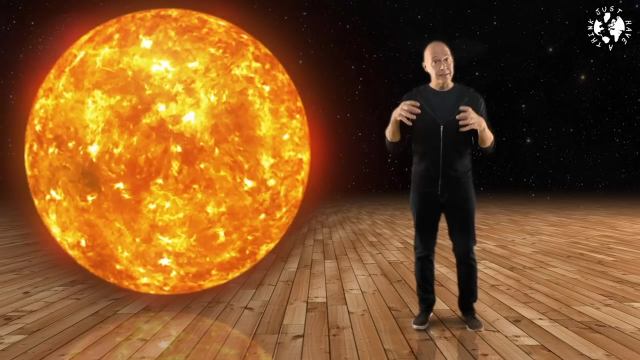 Atomic nuclei all have a positive charge, which ordinarily means that they repel each other, just like when you try to push the same ends of two magnets together. But the sun is also extremely big. You can fit a million earths inside it and that enormous mass creates enormous 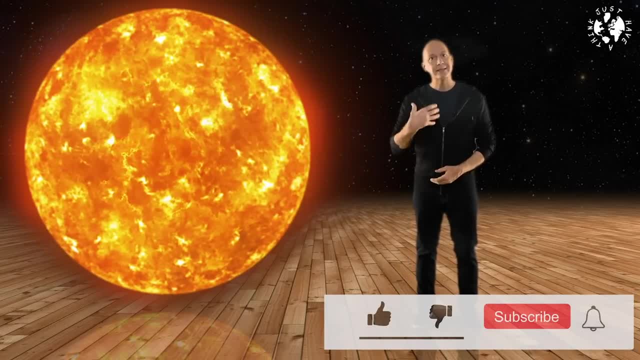 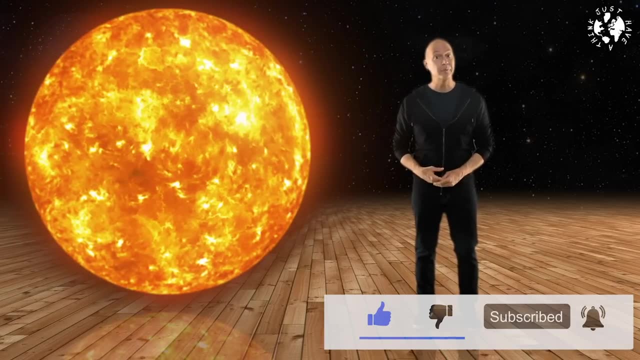 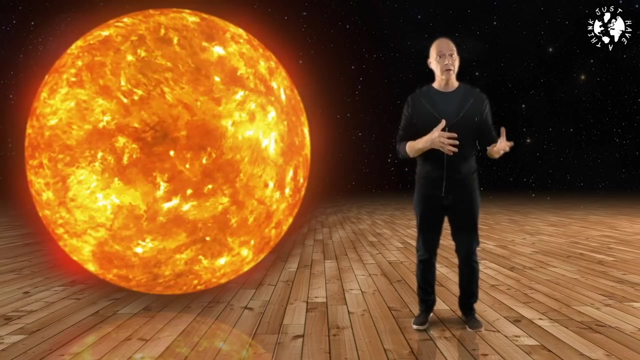 pressure- enough pressure to force those nuclei together, creating heavier elements and releasing really quite mind-boggling amounts of energy in the process. Scientists have been trying to replicate that process on earth for decades. Arguably the two best funded and most competitive inventions today are called tokamak and stellarator. They're both examples of what's. 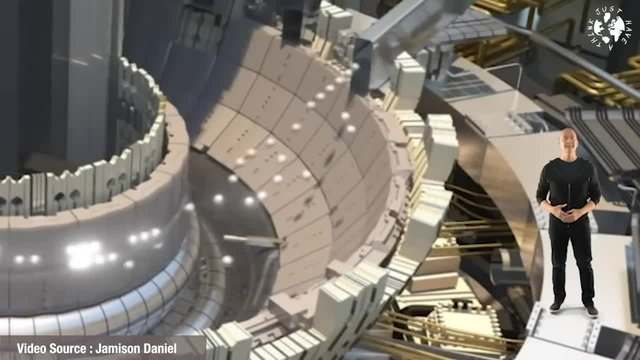 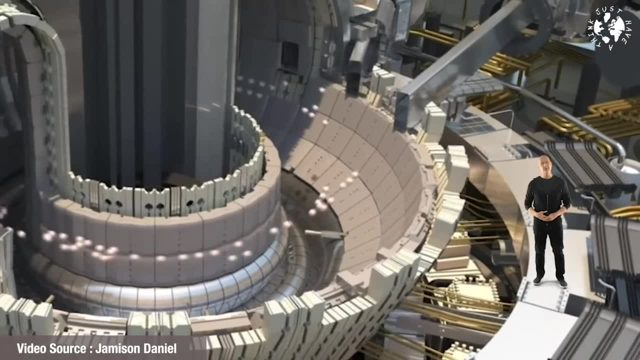 called magnetic confinement technology. This is the inside of the international thermonuclear experimental reactor, or Ita. it's been in development since 1985 and it's the biggest tokamak machine on the planet, at a total of 73 meters or 240 feet in. 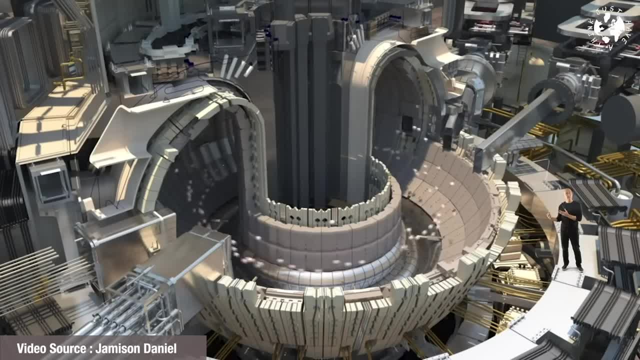 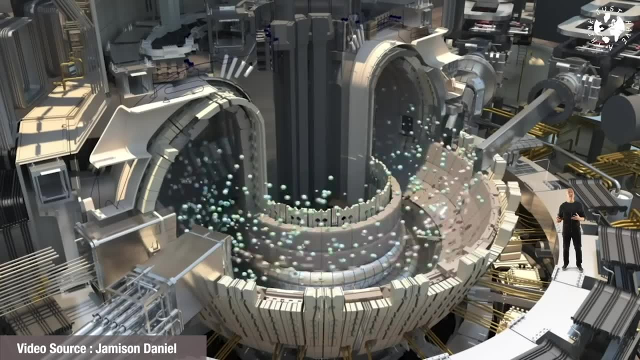 height. It's basically a bunch of incredibly strong magnets that contain a huge donut shaped stream of hydrogen plasma. The plasma gets compressed by the magnets until the nuclei fuse together and release their energy. but getting plasma up to that required temperature and keeping the streams of 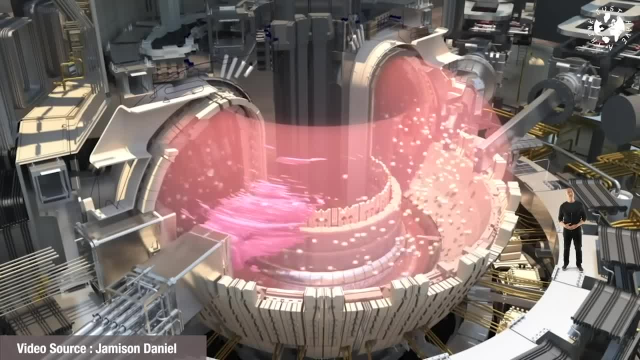 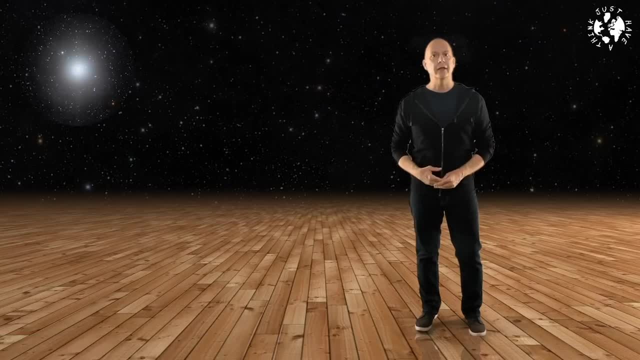 plasma in place long enough for the reactions to take place is extremely challenging and one of the main reasons why the technology hasn't yet come to fruition. There are other tokamak devices being developed around the world, including a UK firm called Tokamak Energy that achieved a plasma. 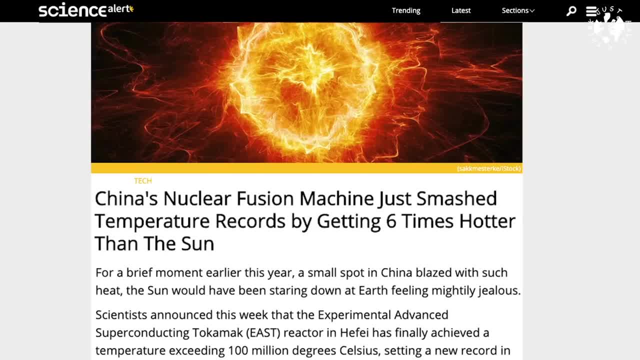 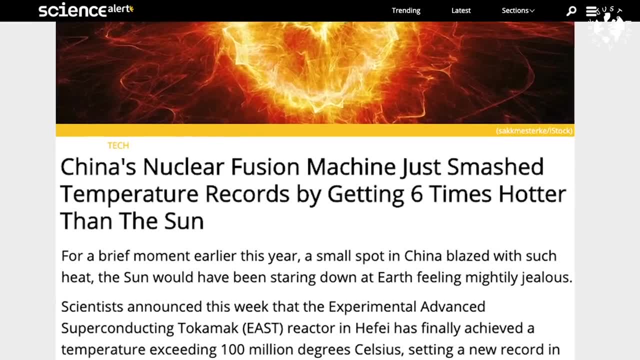 temperature of 15 million degrees in 2018, and another device in China called the Experimental Advanced Superconducting Tokamak, or EAST, which since 2016 has been capable of reaching the elusive 100 million degree target, albeit for a very fleeting amount of time. Stellarator reactors. 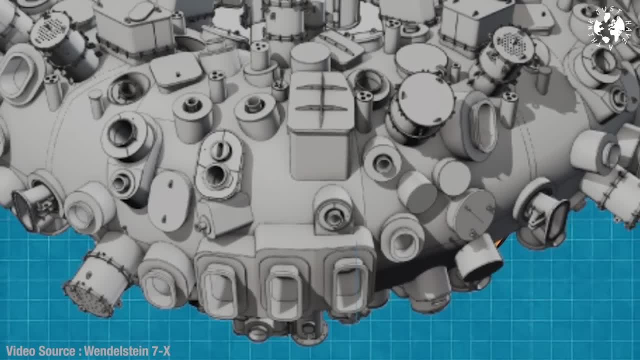 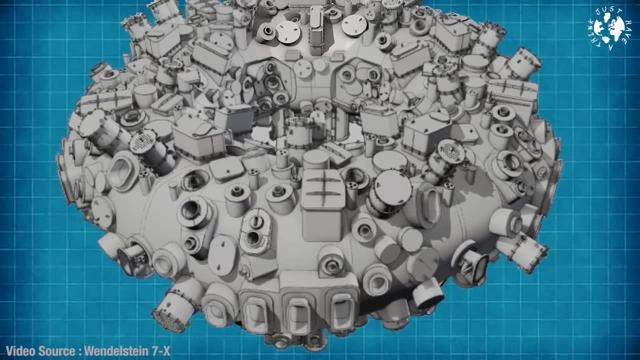 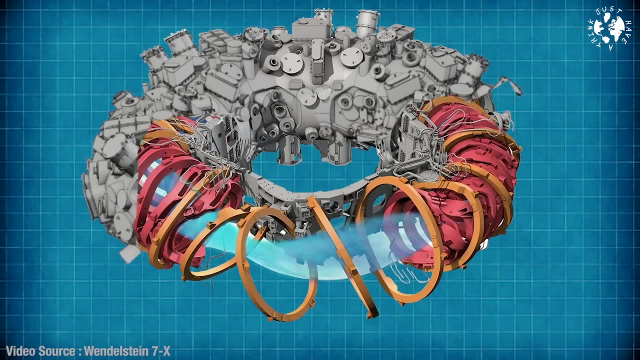 fall under the same category as tokamak devices, but these things represent magnetic containment technology with a twist. quite literally, That big chunk of hardware I was standing in at the start of the video forms just one element of this machine. If we open it up, you can see the weird twisty shape of its vacuum chamber and 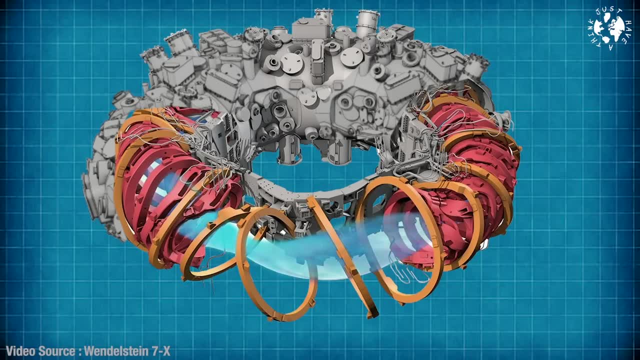 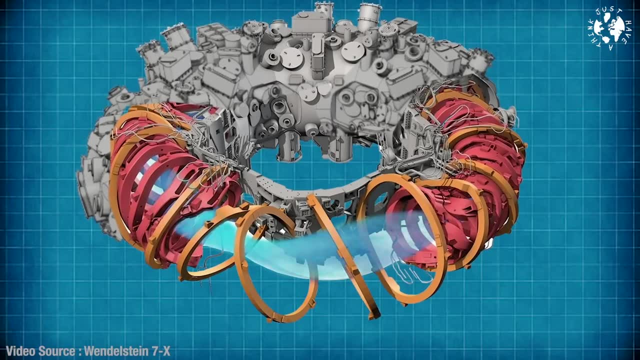 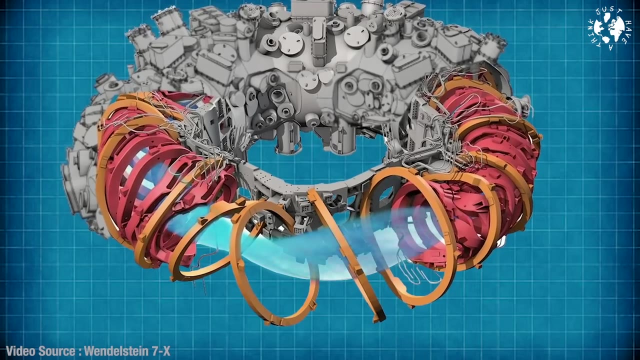 containment magnets, a shape so incredibly complicated that it had to be designed on a supercomputer at the Max Planck Institute in Germany and welded together by precision computer guided robots. There are 50 magnet coils in here, each containing over a kilometer of superconducting cable weighing six tonnes. The idea behind these incredibly intricate twists: 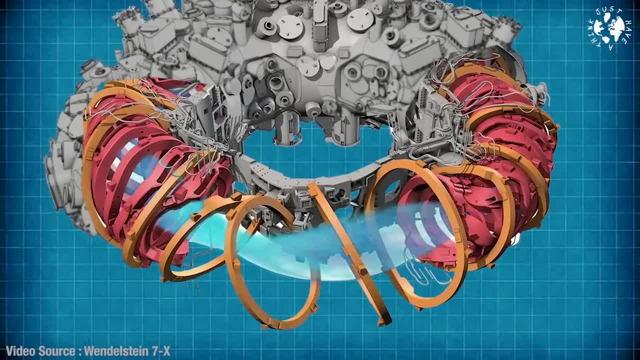 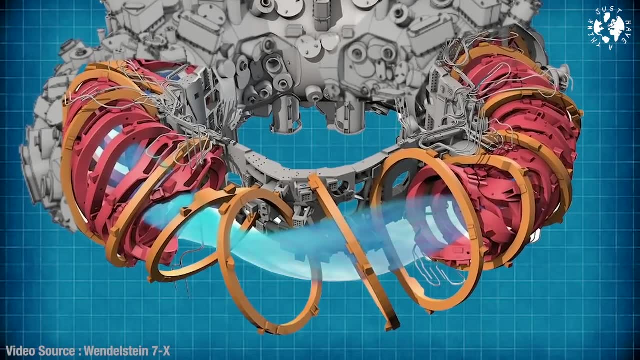 and turns is to overcome a problem encountered in the standard tokamak doughnuts. Inside those more simple shapes, the magnetic field is stronger in the center of the doughnut and weaker on the outer rim. That imbalance causes particles to drift off course and hit the wall of the 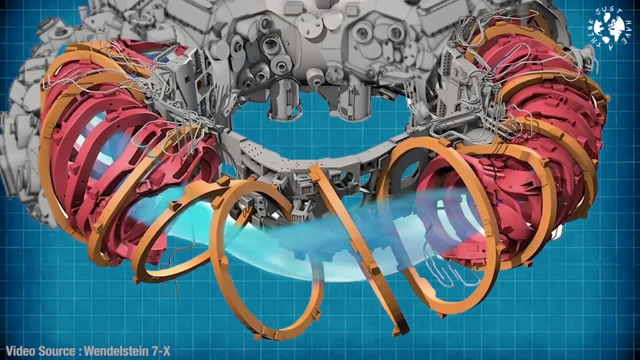 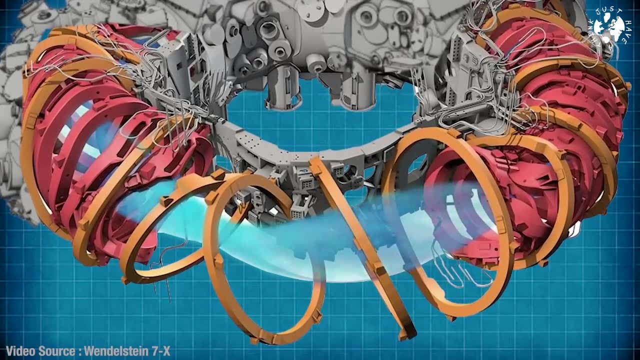 containment chamber, and once that happens, your reaction is over. The stellarator's contorted shapes add a twist that forces particles through regions of high and low. This is the reason why the magnetic fields of the plasma are so close together and the effects of the two cancel each other out. And that keeps the plasma in place so precisely that the reaction tends to be much more reliable. But fundamentally, both these technologies rely on the brute force of enormous energy inputs to raise temperatures to levels that are about seven times higher than the center of the sun. 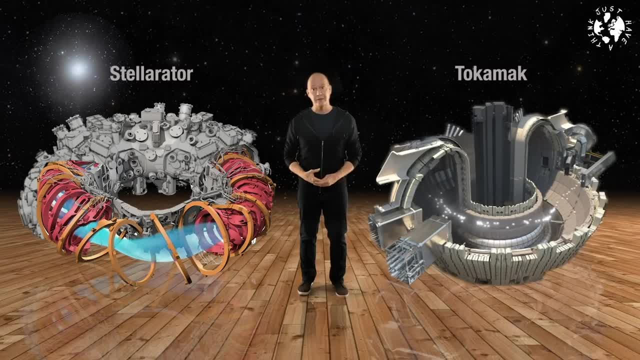 Reaching and maintaining those conditions generally requires more energy than the reaction itself generates. There have been one or two breakthroughs where a net positive energy result has been achieved, But that's not the end of the story. I hope you've enjoyed this video. 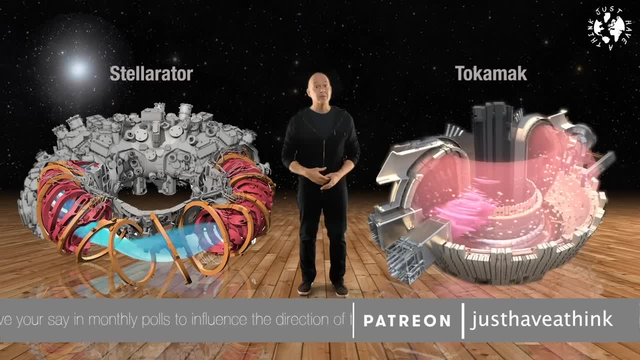 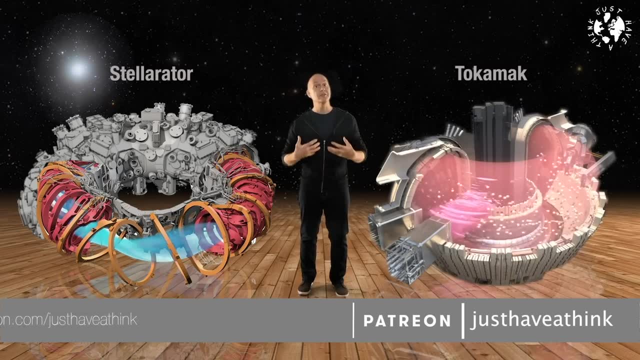 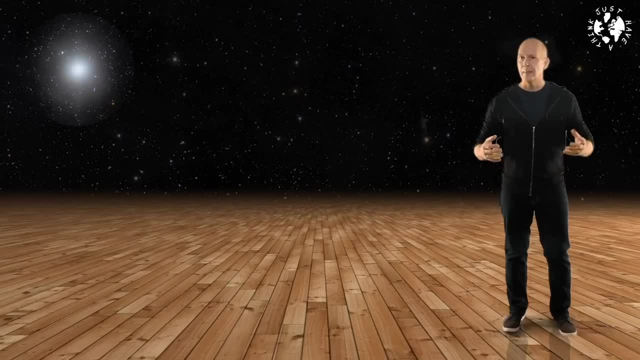 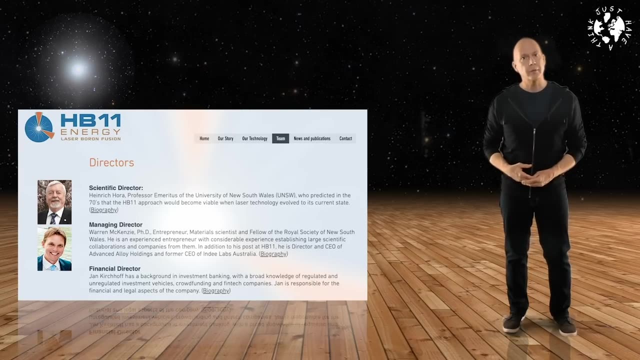 ultimate solution to everlasting, unlimited energy, And that's where our Australian friends come into the picture. The company called HB11 Energy is the culmination of decades of research by emeritus professor Heinrich Hora of the University of New South Wales. On the 21st of February 2020, the company 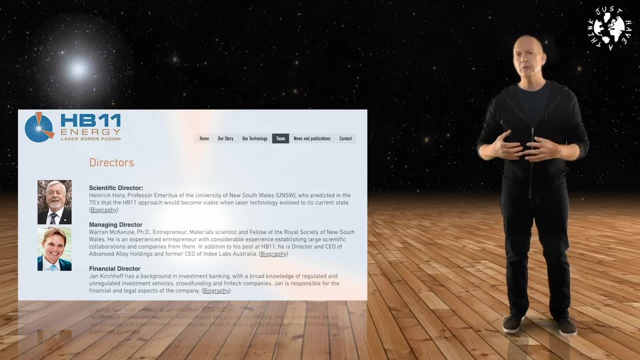 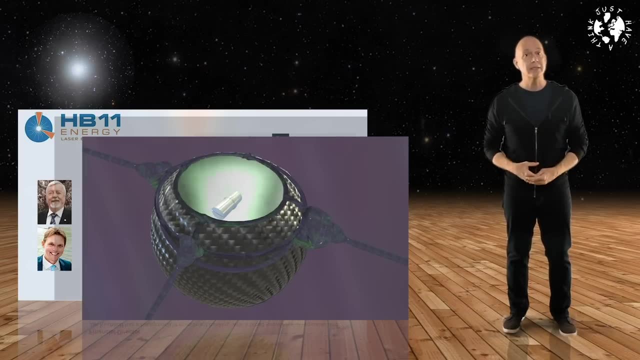 announced that it was ready to launch the HB11.. The HB11 was designed by HB11,, a company that has been working on a series of patents in Japan, China and the USA that protect what it claims is a unique solution to the conundrum of nuclear fusion. The company describes the design as a largely empty. 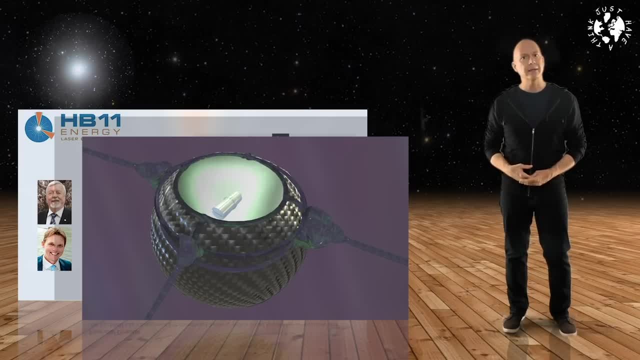 metal sphere, where a modestly sized fuel pellet made up of hydrogen and boron-11 is held in the center with apertures on different sides for two lasers. One laser establishes the magnetic containment field for the plasma, and the second laser triggers what the company call an avalanche. 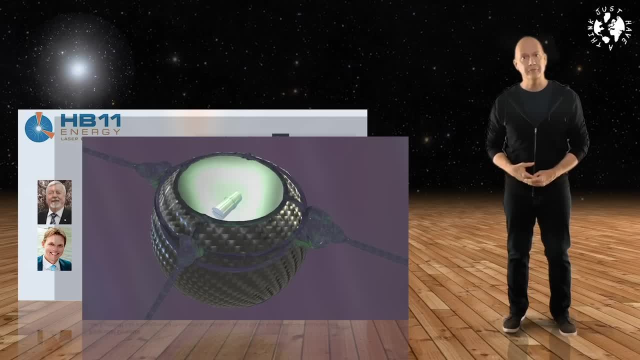 of energy. This is the whole second category of research that sits alongside the magnetic confinement technologies we looked at just now, and that category is called inertial confinement. But, as HB11's managing director, Dr Warren McKenzie, clarifies in an interview with Loz Blaine for the 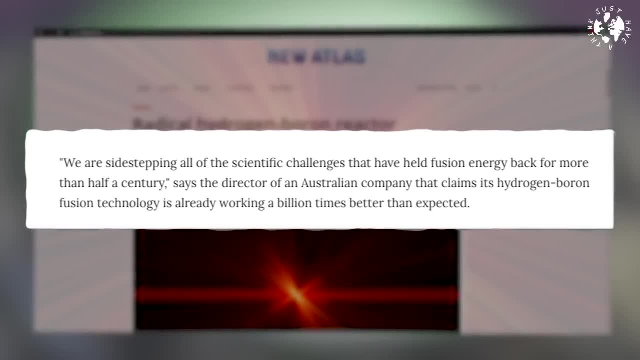 tech website New Atlas, we are sidestepping all the scientific challenges that have held fusion energy back for more than half a century. He says that, unlike other nuclear fusion technologies that simply aim to produce energy- to heat up water, to drive steam turbines- in exactly the same way as nuclear fission or fossil fuel power stations do today, 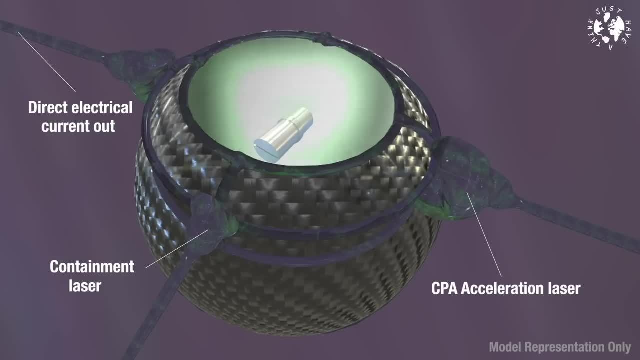 the HB11 concept will directly generate electricity with no steam turbines required, and they claim their experimental system is already working a billion times better than expected. A lot of fusion experiments are using lasers to heat things up to crazy temperatures, says McKenzie. We're not. We're using the laser to massively accelerate the hydrogen through the. 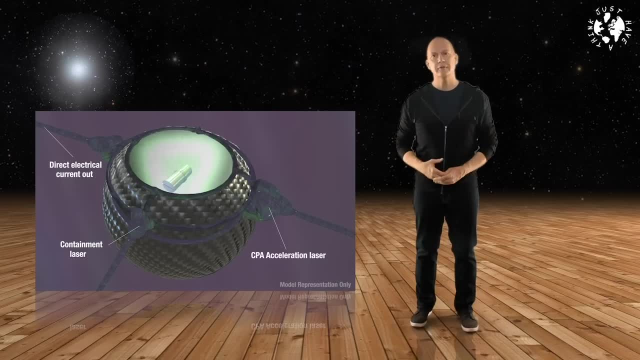 boron sample using non-linear force. He explains that the fusion of the hydrogen and boron creates helium atoms. Those helium atoms are naked, which means they don't have any electrons, and that lack of electrons is a product of HB11's reaction. It means the helium atoms have a positive charge. 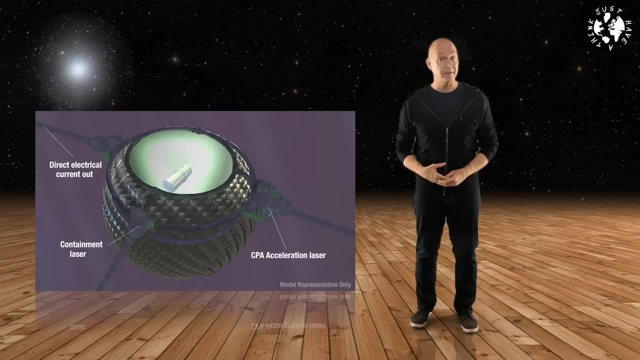 which HB11's machine harnesses, to create a current that can be used directly. The lasers use a technology called chirped pulse amplification, or CPA, developed in the mid-80s by Donna Strickland and Gérard Moreau of the University of Rochester in New York. The technicalities of that technology. 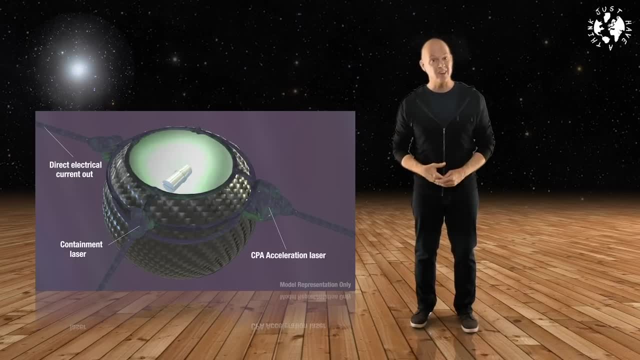 are way outside the scope of this video, But essentially it's a way of amplifying tiny laser pulses up to enormous power levels. We're talking petawatts of energy here, which is a lot of zeros. My vacuum cleaner is rated at about one. 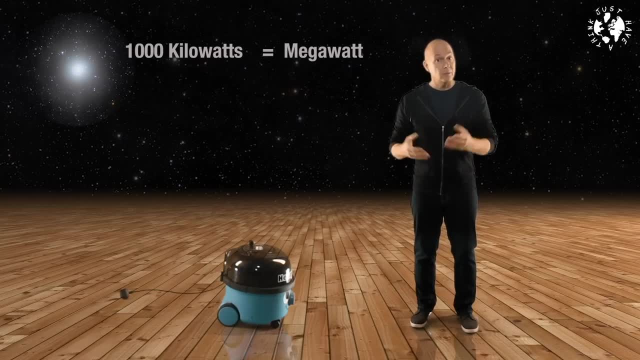 kilowatt. A thousand of these would be a megawatt. A thousand megawatts is a gigawatt, a thousand gigawatts is a terawatt and a thousand terawatts is a petawatt, which is just a ridiculous amount. 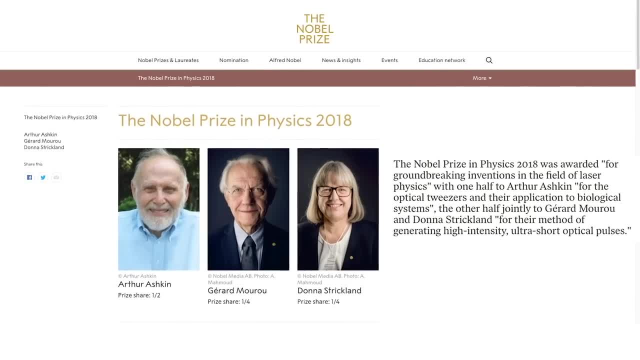 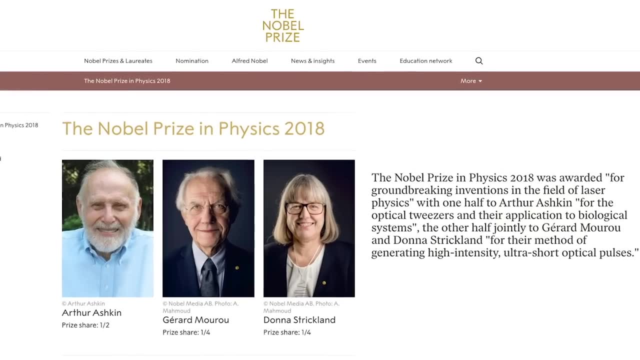 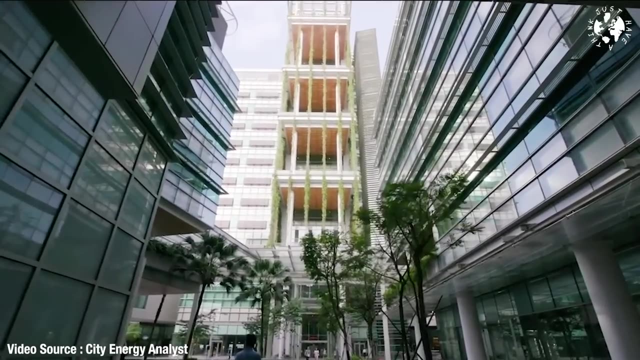 of energy. Anyway, the development of CpA earned its inventors the 2018 Nobel prize in physics, so it was a big breakthrough, and it means that HB11's reactors would be much smaller and simpler than the high temperature fusion generators like tokamak, and stellarator Dr McKenzie says that their generators would be. 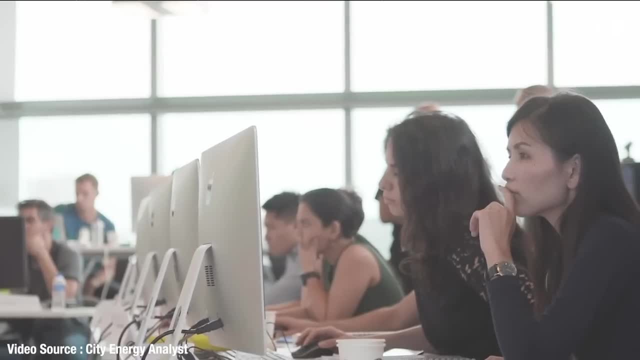 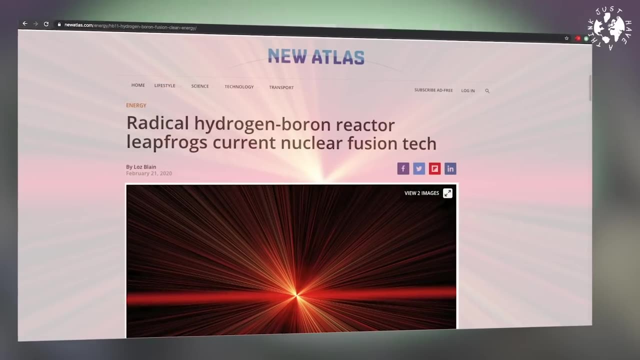 compact, clean and safe enough to build in urban environments, with no nuclear waste involved, no superheated stream and no chance of a meltdown. The father of the technology, Professor Heinrich Hohrer, is extremely optimistic about HB11's achievements. 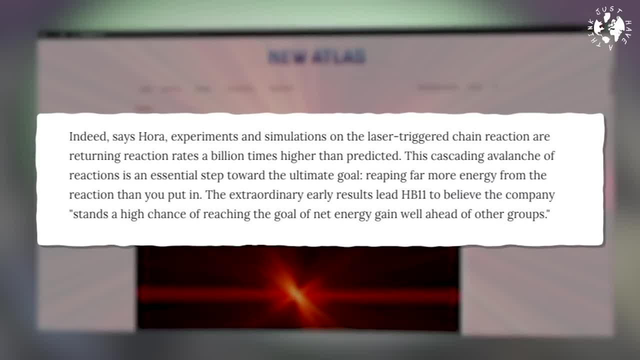 Experiments and simulations on the laser-triggered chain reaction are returning reaction rates a billion times higher than predicted. This cascading avalanche of reactions is an essential step toward the ultimate goal of reaping far more energy from the reaction than you put in, which means HB11 stands a high chance of reaching the goal of net energy gain well ahead of the. 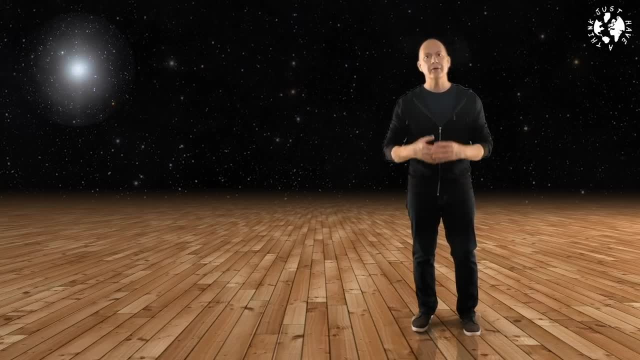 other groups. What's really amazing, said Dr McKenzie, is that Heinrich Hohrer envisaged and described this technology way back in the 1970s. It's only possible now because the brand HPA lasers are capable of doing it. So let's cut to the chase then. When's it going to be ready? 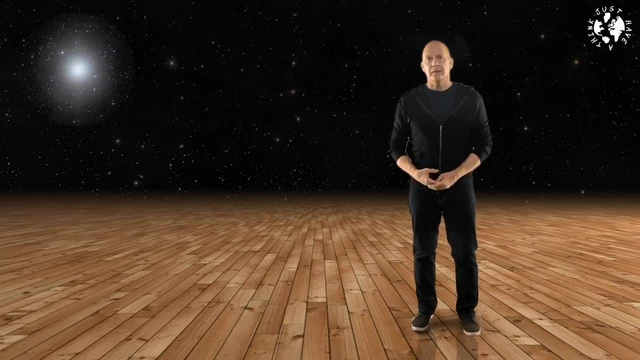 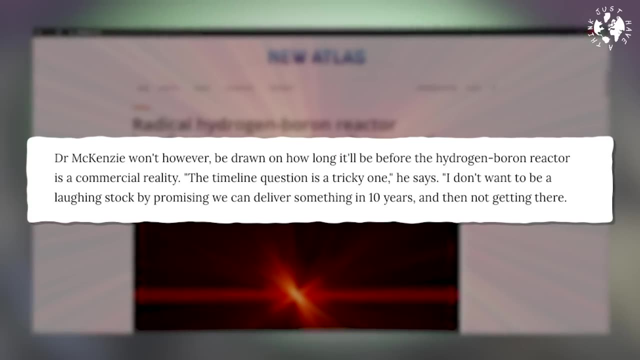 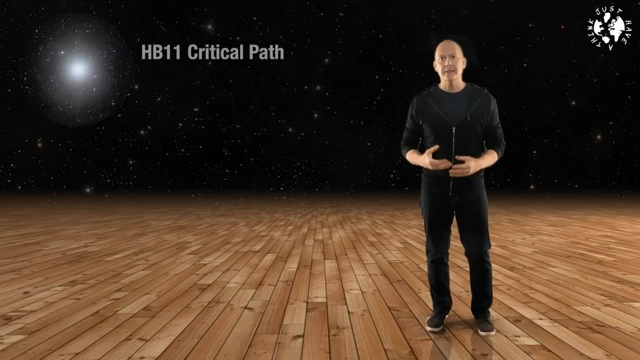 for commercial scale rollout. Yeah, let's check back with Dr McKenzie again. The timeline question is a tricky one, he says. I don't want to be a laughingstock by promising we can deliver something in 10 years and then not getting there. First step, he says, is setting. 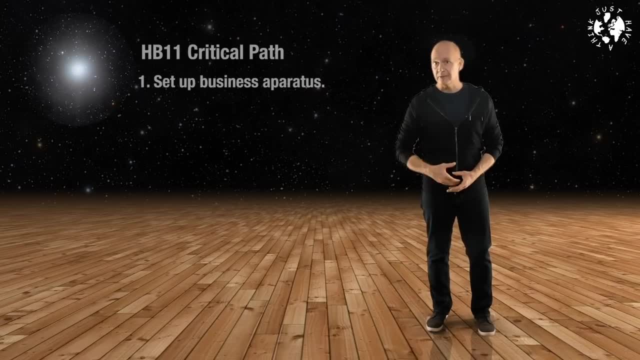 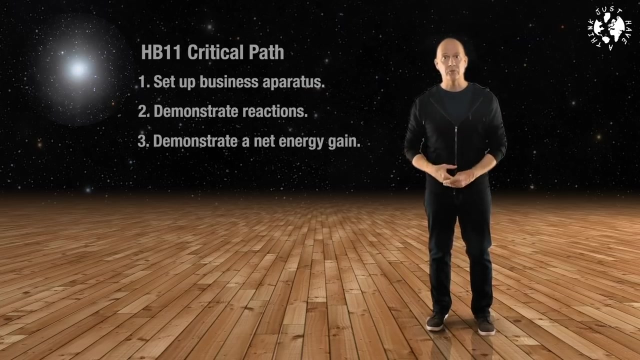 up camp as a company and getting started. The first milestone is demonstrating the reactions, he said should be easy. Second milestone is getting enough reactions to demonstrate an energy gain by counting the amount of helium that comes out of a fuel pellet. when we have those two lasers working together, That'll give us all the science we need to engineer a reactor. 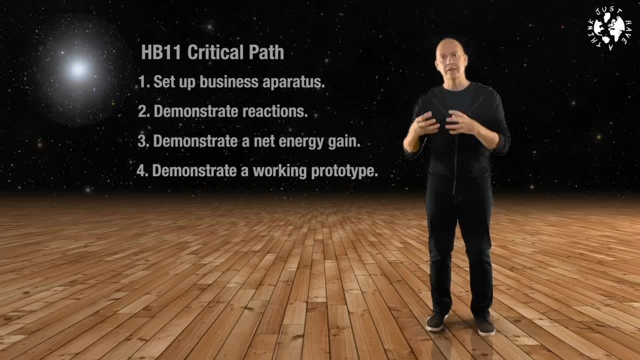 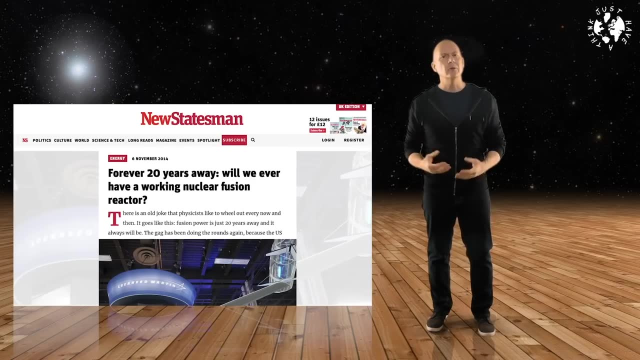 So the third milestone is bringing that all together and demonstrating a reactor concept that works. So that cliche I mentioned earlier, you know, the one about nuclear fusion always being 20 years away, That one, yeah, Well, it looks like.